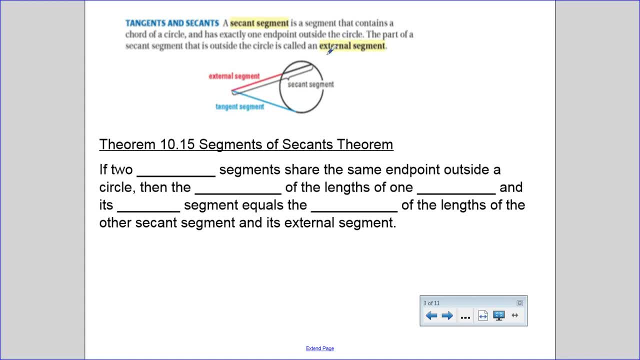 circle is called the external segment, which makes it external means outside. So this piece here that's in red, that's the external segment and it's part of the secant segment. And then here we have our tangent segment. So theorem 10.15 says segments of secants. theorem says: if two secant 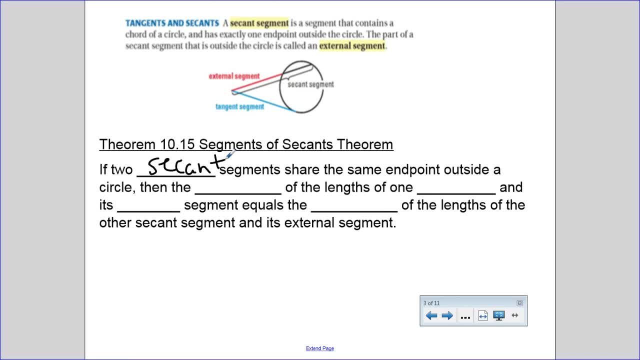 segments share the same endpoint outside a circle, then the product of the lengths of one secant segment- so secant segment, really squishing it in there- and its external segment equals the product of the lengths of the other secant segment and its external segment. 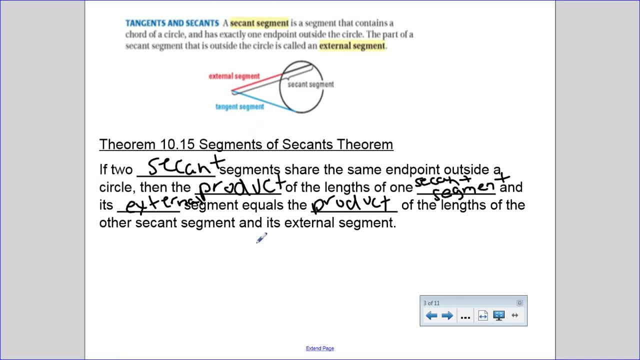 Now, if you're saying what the heck does that mean? What the heck does that mean? What the heck does that mean? Well, let's see how I do my circle drawing. So here's a circle And say I have here's one secant. 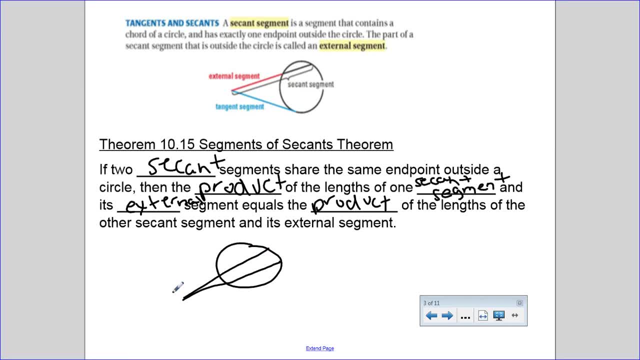 And here we go. We'll have another one here And I'll try labeling them. So if this is A, B, C, we'll call this D and E. What this is saying is this external segment here, So A B times the whole secant segment. 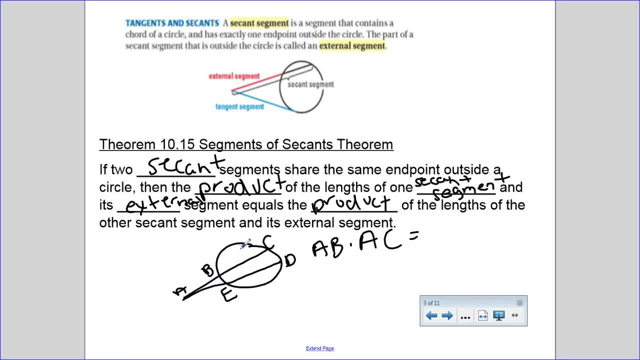 So A B times A C. So the outside piece times the whole thing would be equal to the outside piece of the other one times the whole thing. So external times whole thing. So piece times whole thing is equal to piece times whole. thing. 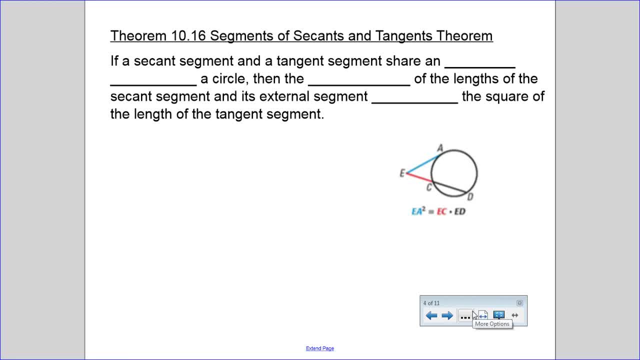 Again pretty cool. Theorem 10.16, segments of secants and tangents. theorem. Say that three times fast. If a secant segment and a tangent segment share an endpoint outside, so endpoint outside a circle, then the product. 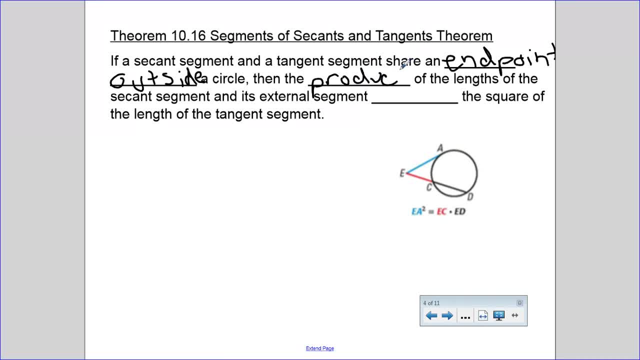 of the lengths of the secant segment and its external segment equals the square of the length of the tangent segment. So in this one, as you see here, here's our tangent and here's our secant. But this is saying, as it's labeled here, that tangent segment E A squared. 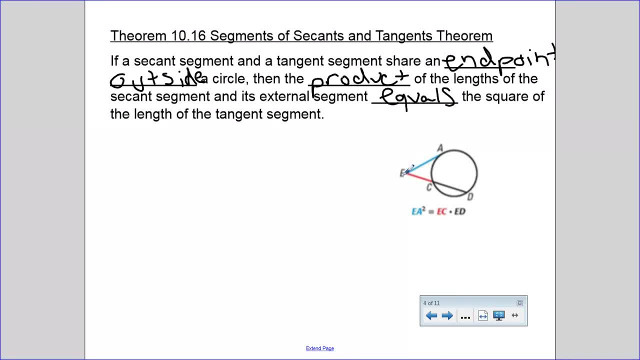 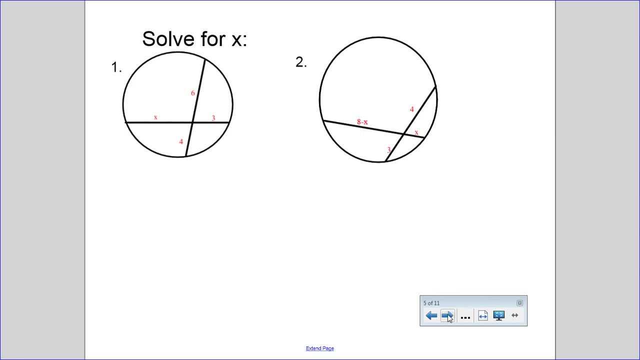 is equal to E C times the whole thing. So the part times the whole is equal to this part squared. All right, so that's three new theorems. Let's see how it works. All right, solve for X. Well, this was our first theorem: 10.14.. 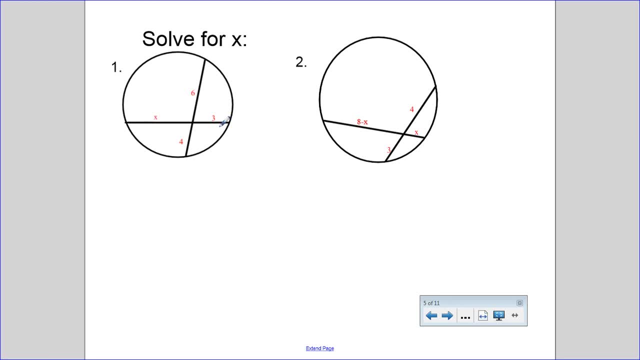 So this one for number one, we say: okay, the two pieces three times X equals six times four. So three X equals 24.. Therefore X must equal eight. Here let's have some fun with quadratics. So the small piece of four times three is equal to X times eight minus X. 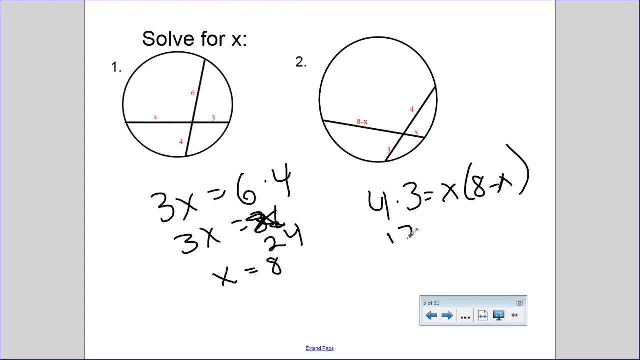 Okay, 12 equals distribute eight X minus X squared. Now, normally I would move the 12 over here, but see that negative sign in front of the X squared. I don't want that, so I'm going to move everything to the other side. 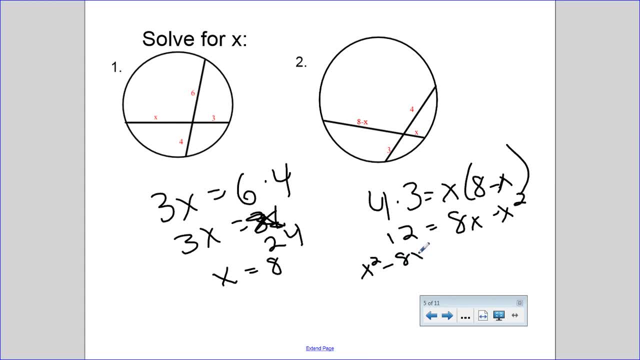 I get X squared minus eight. X plus 12 equals zero, because when we're factoring it has to be set to equal first, so we can find all values for X. Now, remember, I'm going to find the factors of 12 that have a sum of negative eight. 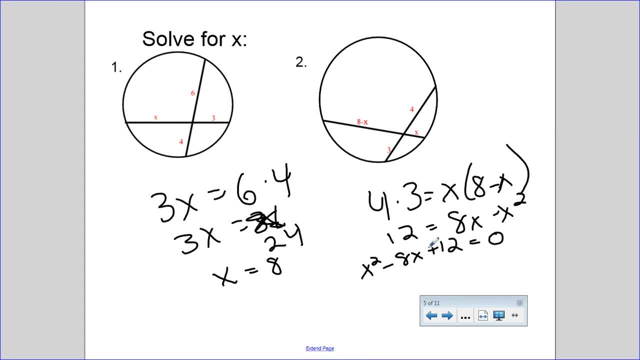 If you both right, they both have to be negative to get a positive here when I multiply. So I get X minus six, X minus two equals zero. Now I've set this equal to zero. that equals to zero. What you should get is that X could equal six or X equals two. 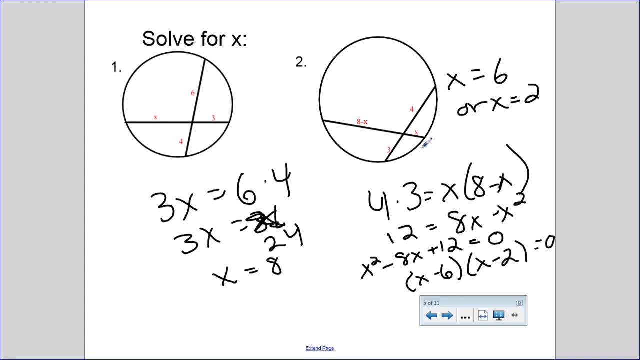 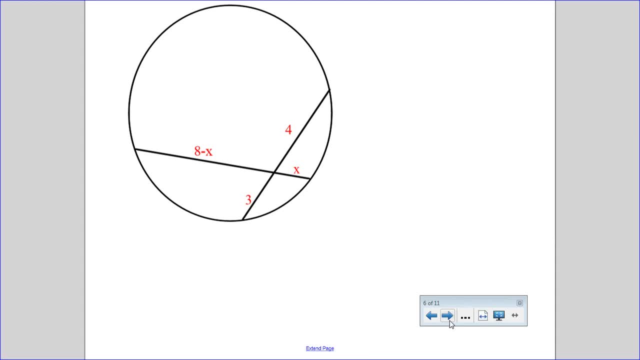 Both would work. Yeah, I have no negative values here. All right, this one we can skip, because we actually just did it. It's a double. All right, now we're looking at our external pieces. So for this one, now this is telling us that 12 is the measure of the whole thing. 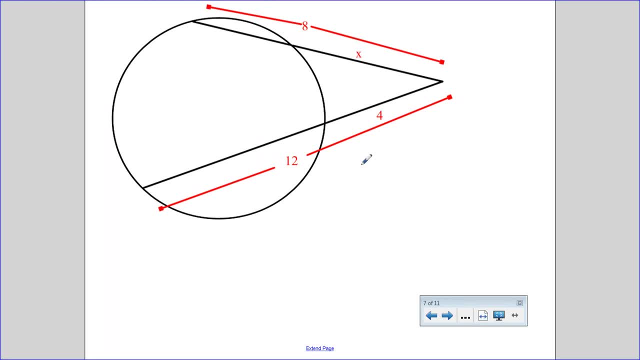 eight is the measure of the whole thing in this one, okay, So remember this is where piece times whole, piece times whole. So this one would be X, eight times X, so the whole times the piece, so the whole is four times 12.. 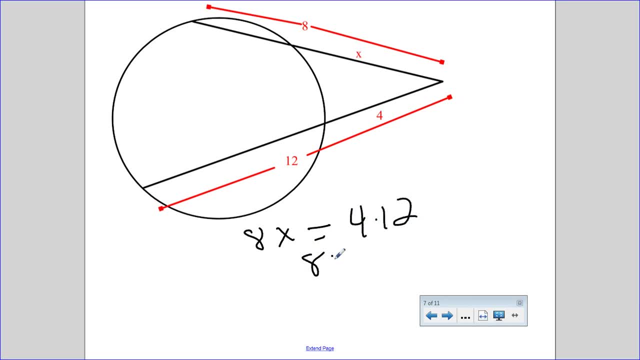 So we get eight. X equals 48,, X equals six, Okay, Okay, another one dealing with our pieces. Oh, this time it's not telling us the whole, So for this piece, the whole would be six plus X. Okay. 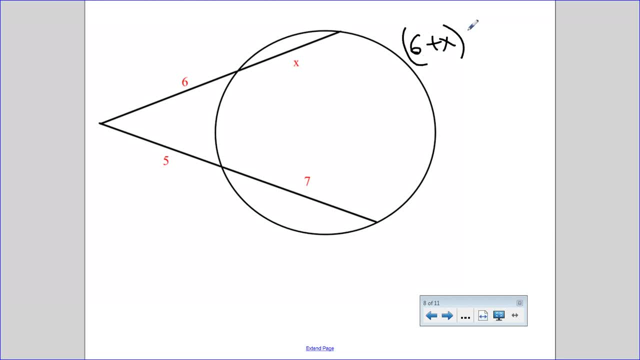 So this one would be X times the piece, which is six must equal five plus seven, which is 12, times the outside five. all right, So now I'm going to distribute and I'm going to get 36 plus six times X equals 60.. 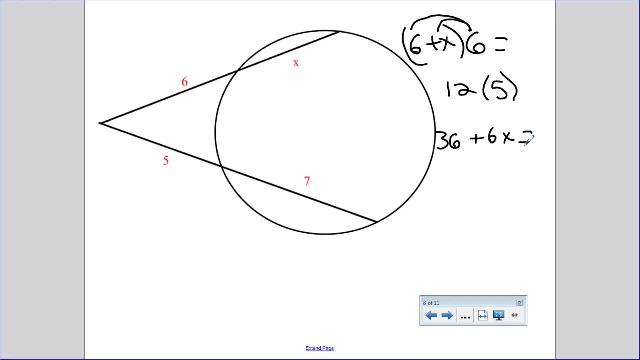 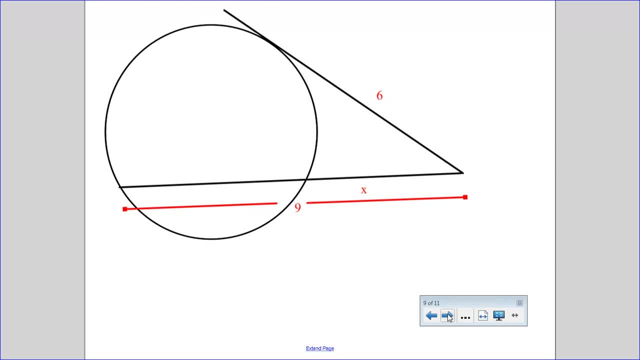 All right, All right. so this piece squared. so 6 squared equals piece times whole. so 9 is the whole x, so 36 equals 9x, x equals 7.. All right, this one, same kind of setup, right, This squared. 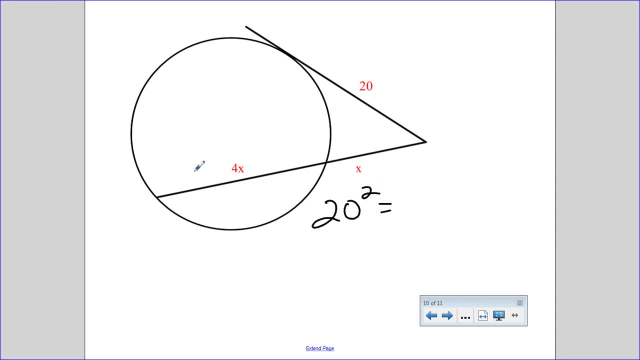 so 20 squared equals well, the whole piece would be 4x plus x, right? because it's not indicating that either one of these is the whole. it's saying these are each the pieces, right? So 4x plus x times the outside piece, right? So I can say 400. 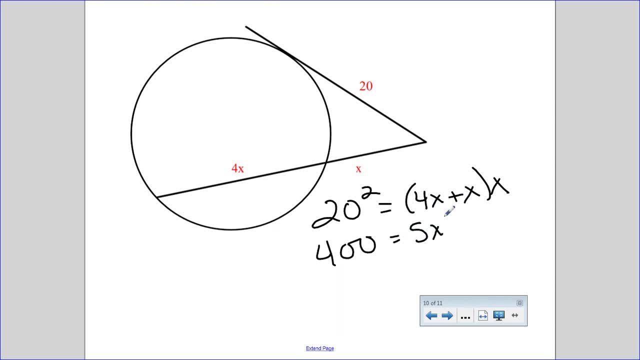 equals 5x right in combined like terms times x. so 400 equals 5x squared right. So from here you want to divide by 5, right, and I'm going to move it this way. and I'm going to divide by 5, and I'm going to move it this way. 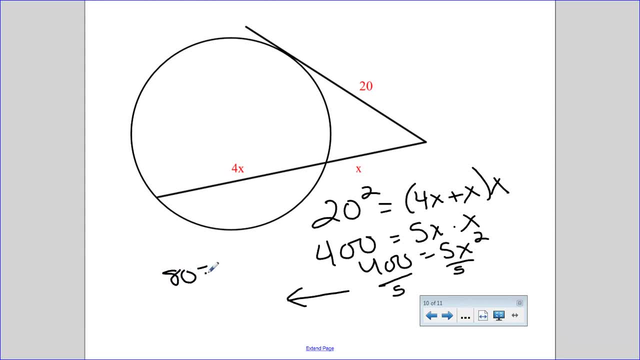 and I'm going to move it this way. and I'm going to move it this way and I get 80 equals x squared. Now you know, I like my square roots in exact form. I'm going to take the square root of both sides and I get x equals. well, 80 is 16 times 5.. 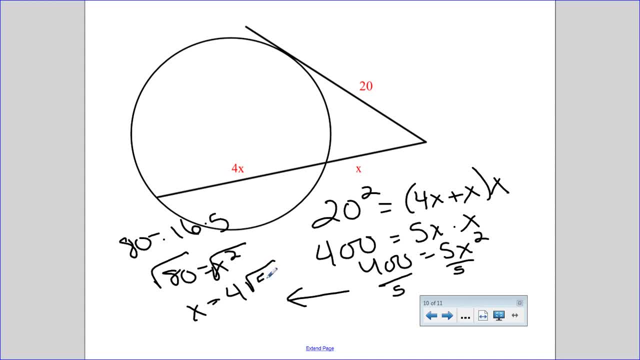 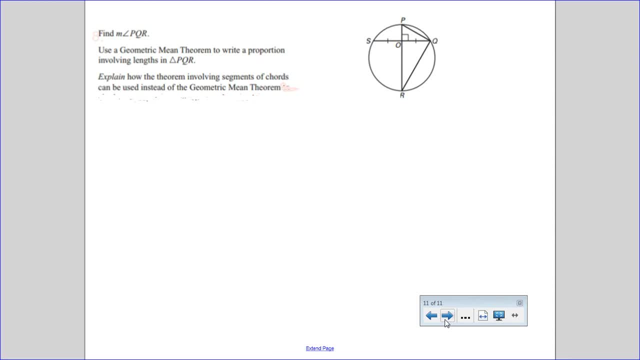 So I'm going to say it's 4 square root of 5.. And now let's do some deep thinking. We want to find the measure. we'll start with finding the measure of angle, PQR. Okay, well, I see that PR is the diameter of a circle, right, If this is circle O? 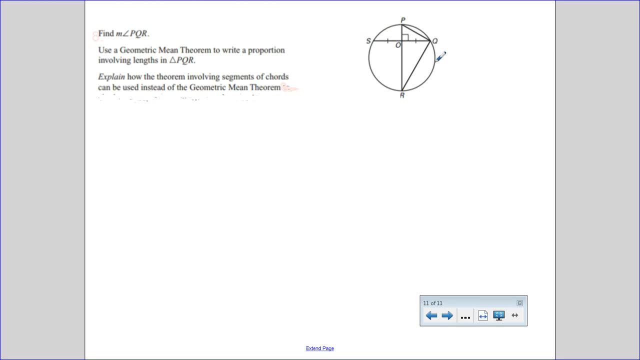 I know it is. it goes through the center. If that's the diameter, then I know this must be a right triangle. So the measure of angle PQR must be 90 degrees, Because that diameter would be the hypotenuse. Alright, the second question it asks is: use a geometric mean theorem to write a proportion. 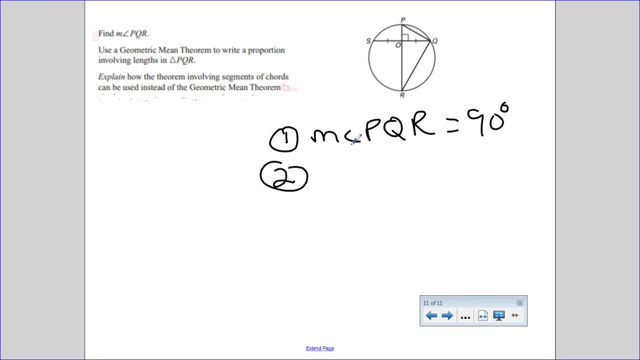 involving the lengths of triangle PQR. You have to remember something from the last unit. Okay, so the geometric mean theorem says: if you have the altitude, you can say that the measure of the leg so OP. you can say that the measure of the leg so OP over that altitude. 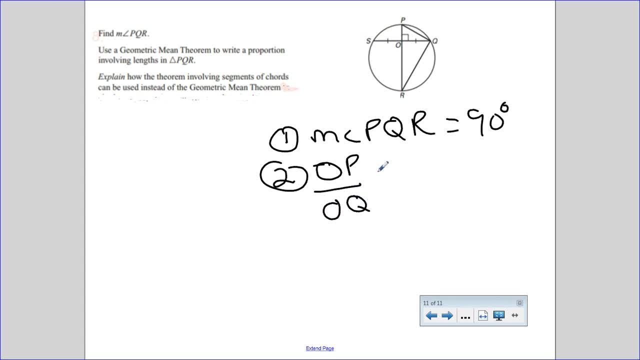 is in proportion to OQ, again over OR? Alright, so now you remember the geometric mean theorem. Here's our proportion, And if you look at it so you're saying let's move over here, OP. so the short leg to the long one of this little triangle is a proportion with this triangle. 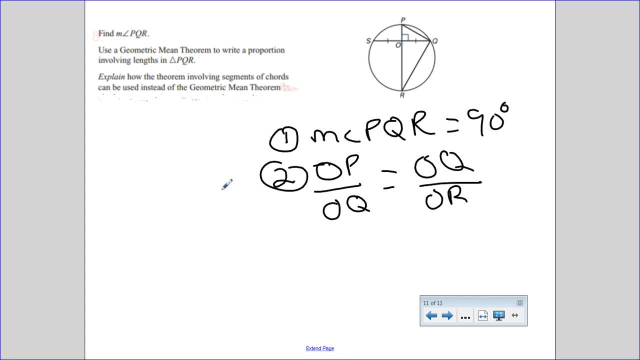 short to the long, OQ to OR. All right, Now I need some room to explain. number three: Explain how the theorem involving segments of chords can be used instead of geometric mean theorem. If you look at your notes, the segment of chords was the first one, So I think it's 10.14.. All right, So these would 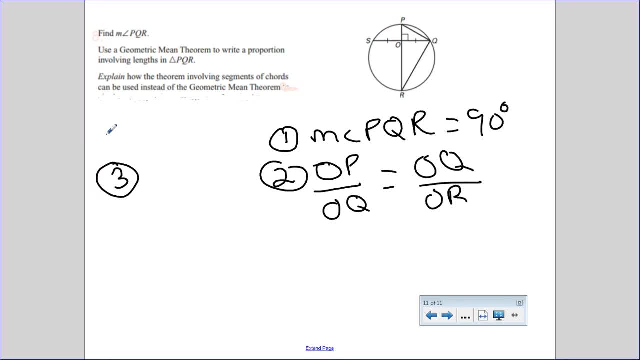 be internal chords. Now, by the segment of chords it says that if I took the products right, OP times OR would have to be equal to OQ, oops, OQ times, OS right the products. Now you're told in the diagram that OQ equals OS, right, They're congruent. 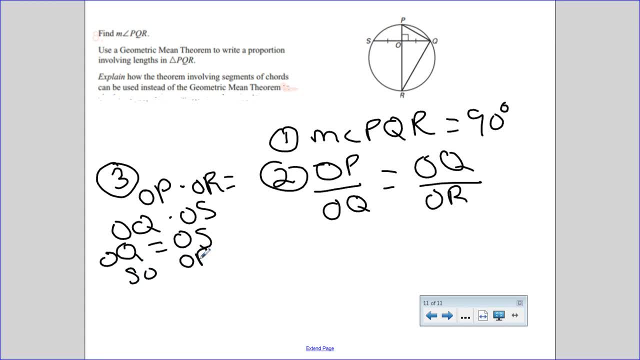 So OP times OR is equal to OQ, squared right. if I were to right, these two would be the same, which would be the same, So that'd be the same if we did the cross products right. If we did took our. 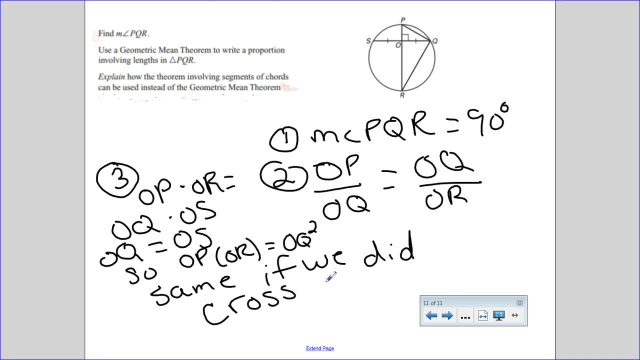 proportion in number two and did cross products, we would get the same thing, All right. So there we go. It'd be the same thing, All right. Well done Here. put a little smiley for Ryan. You're doing awesome. Keep up the good work. You can use the rest of class time.